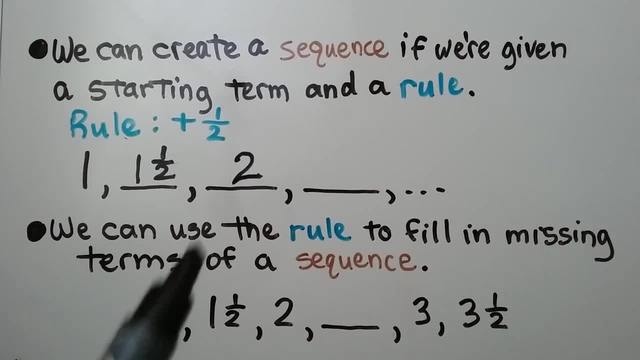 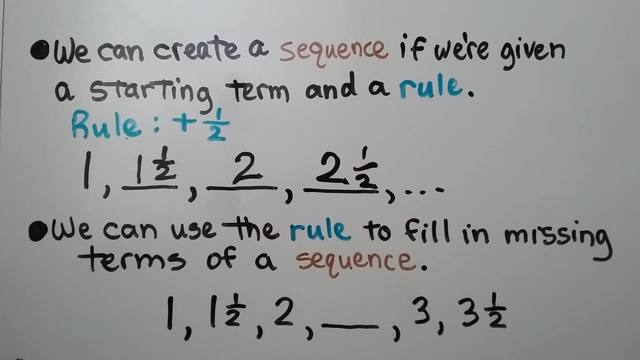 Two whole Plus half again would be two and a half. We can use the rule to fill in missing terms of a sequence. If we know the rule is plus half and it shows two here we know this must be two and a half. 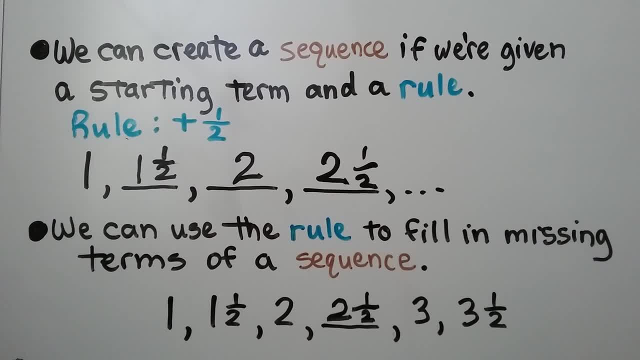 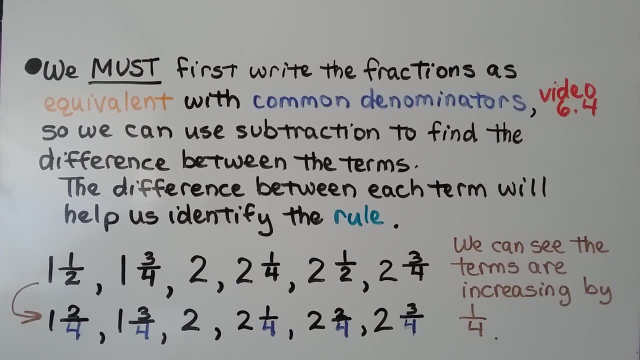 Knowing the rule can help us complete a sequence, or it can help us find a missing term of a sequence. We must first write the fractions as equivalent with common denominators. And again we learned about equivalences, Equivalent fractions and common denominators in 6.4.. 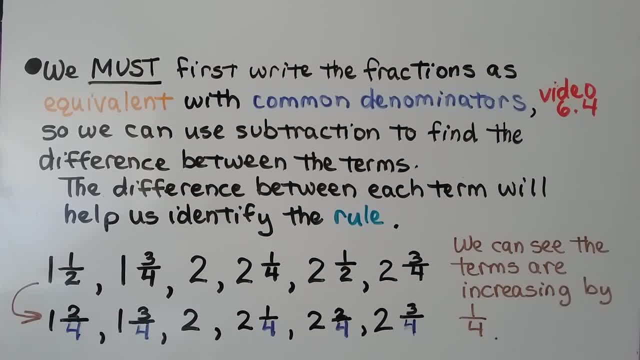 So we can use subtraction to find the difference between the terms And the difference between each term will help us identify the rule. We have one and a half, one and three fourths. two, Two and one fourth. two and one half, two and three fourths. 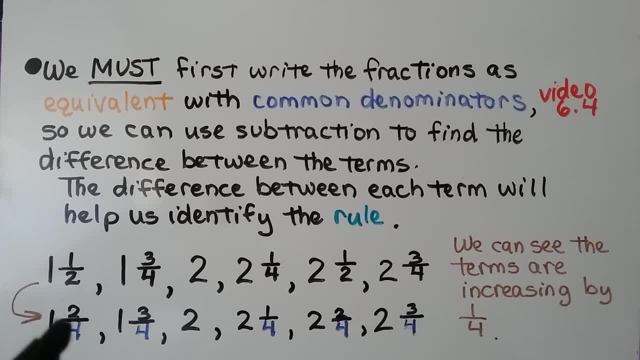 If we write them all with a common denominator, we get one and two, fourths, one and three, fourths, two, Two and one, fourth, two and two, fourths, two and three, fourths, Two and two, fourths, two and three fourths. 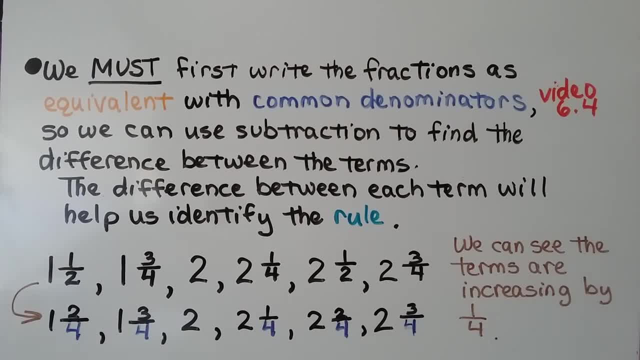 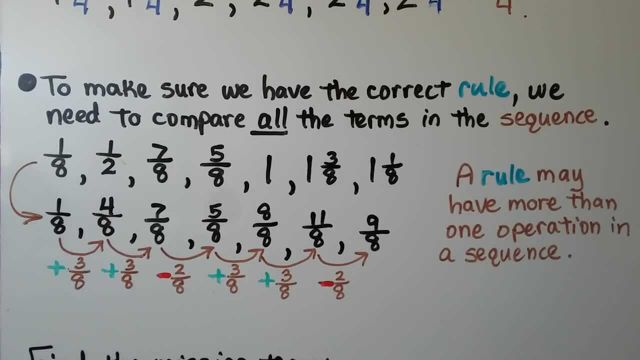 And we can see the terms are increasing by one fourth. To make sure we have the correct rule, we need to compare all the terms in the sequence. We have one, eighth, one half seven, eighths, five, eighths, One, then one and three eighths, then one and one eighth. 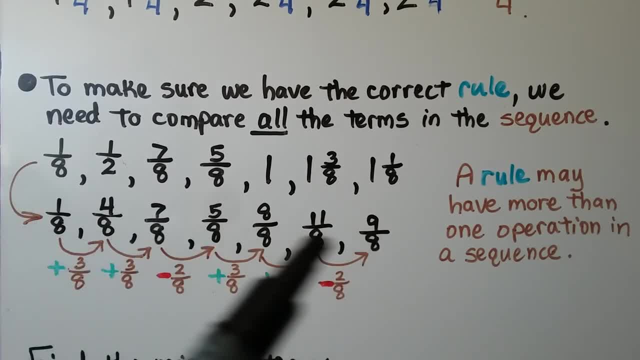 We can see if we give them all eighths as the denominators, the denominators, we have one eighth, four eighths, seven eighths, and then it goes down to five eighths, then it goes back up to eight, eighths. 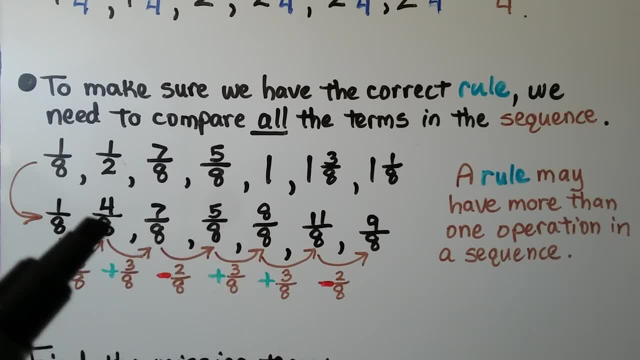 What's happening is we're adding three eighths to get four eighths. we're adding another three eighths to get seven eighths, but then we're subtracting two eighths, Then we're adding three eighths again, adding three eighths again. 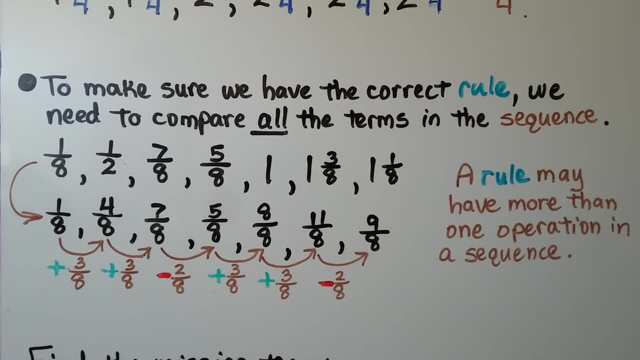 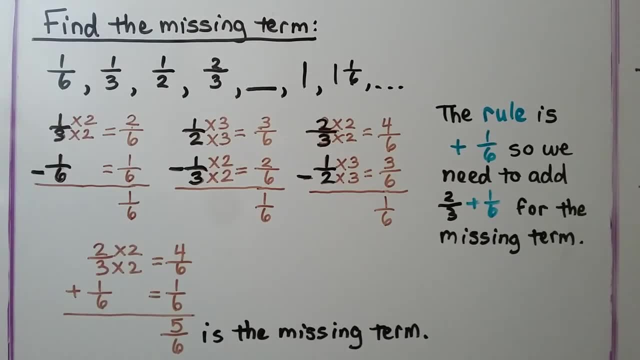 and then subtracting two eighths. So a rule may have more than one operation in a sequence. Here we have a sequence with a missing term. We need to find the missing term. We see the denominators are a six, a three, a two. 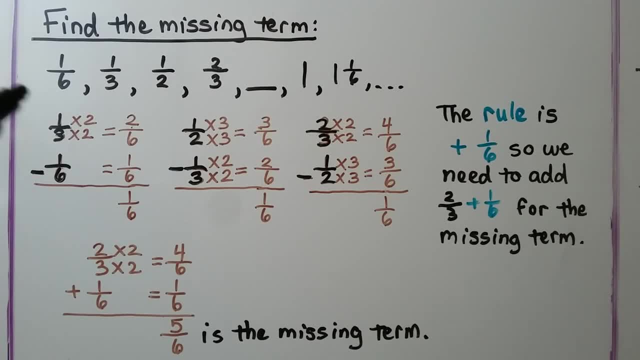 then a three again. This one's got a six. We can give them all a six as a common denominator And we take this term 1- 6, and subtract it from this term 1- 3rd, 1 3rd minus 1- 6,. 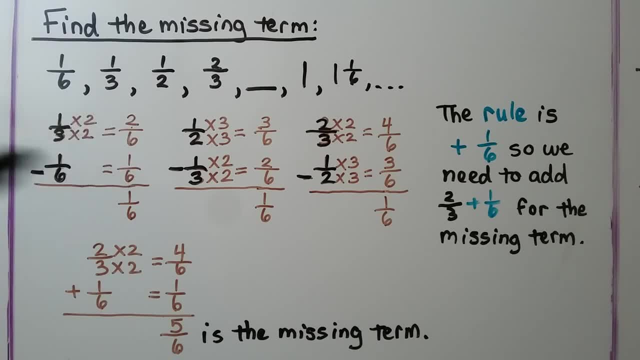 giving them both a six for a common denominator, we get 2, 6 minus 1, 6. That's 1, 6.. Then we take this term as 3, 6.. We multiply the numerator and denominator by three. We get 3, 6 minus 2, 6.. 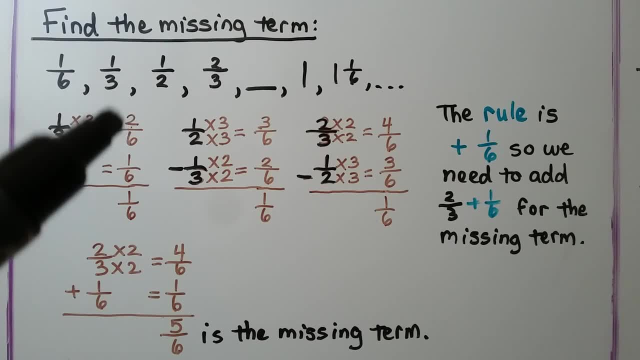 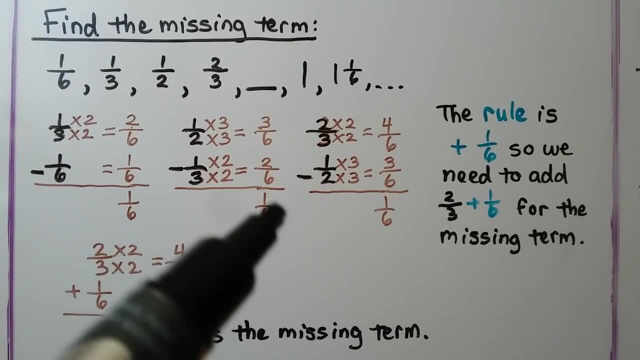 We now know that this 1- 3rd can be written as 2: 6, so we use that for our comparison. 3 6 minus 2: 6 is 1, 6.. So far, the difference is 1: 6th between each term. 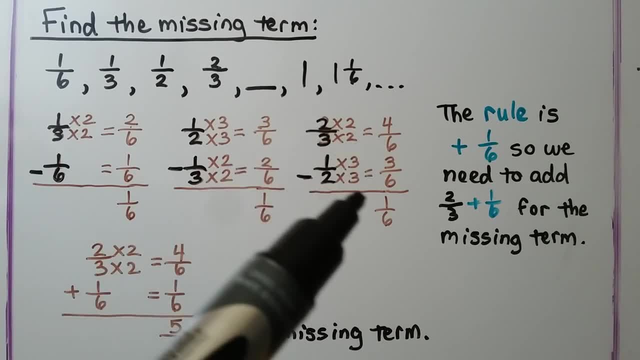 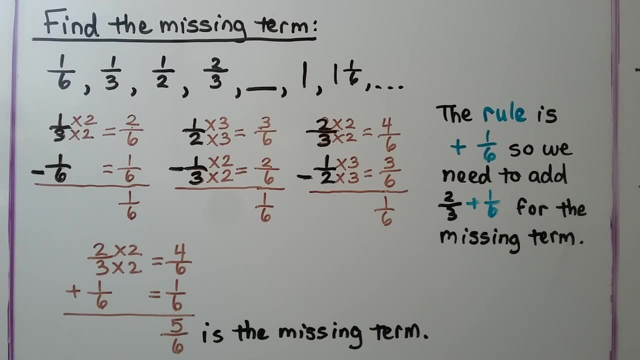 We do 2- 3rds, Which is 4, 6s, And we subtract 3- 6s, This one rewritten with six as a denominator. We get 1, 6. So the rule is plus 1- 6th. 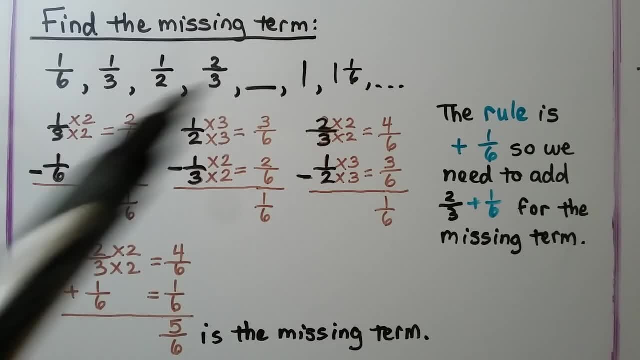 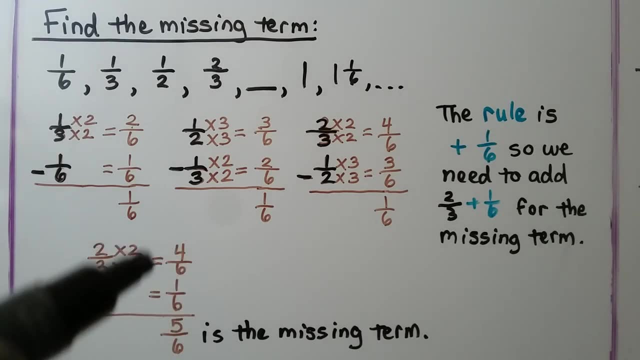 So we need to add 2 3rds plus 1, 6 for the missing term, 2 3rds plus 1, 6.. We give them both six for a denominator, That's 4, 6 plus 1, 6.. 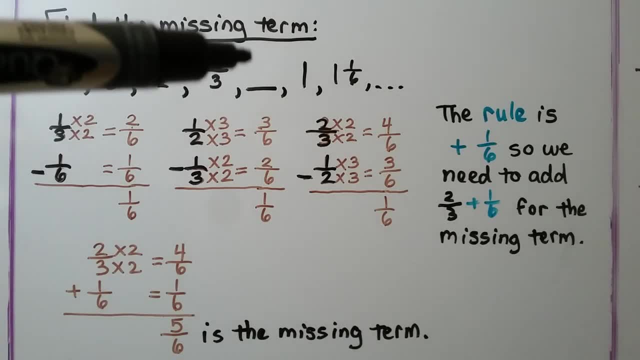 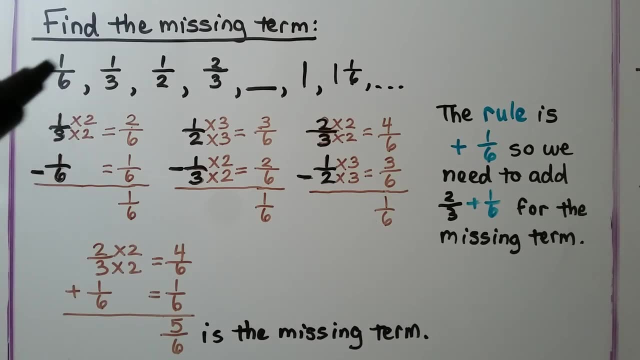 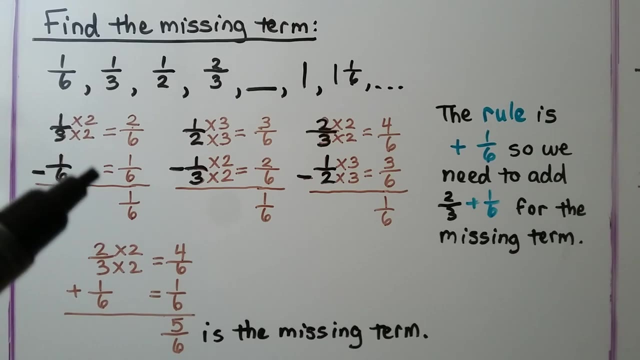 That's 5- 6.. We know that this missing term must be 5- 6ths. We need to subtract the first term from the second term, Then the second term from the third term and the third term from the fourth term. We needed to keep subtracting to find the difference between them. 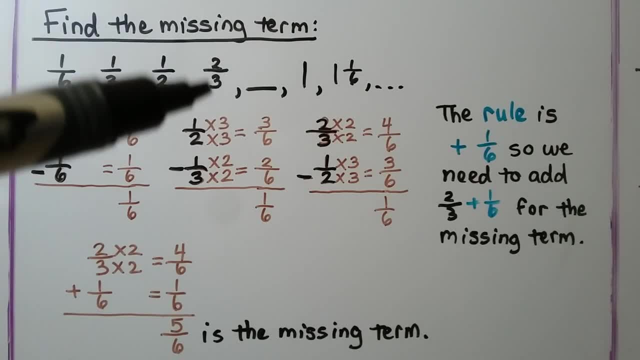 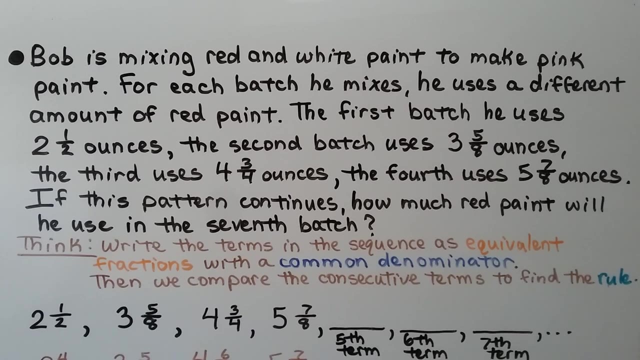 And then, once we did find that difference, we needed to add it to this term to get the next term, Because they're all increasing. Bob is mixing red and white paint to make pink paint. For each batch he mixes, he uses a different amount of red paint. 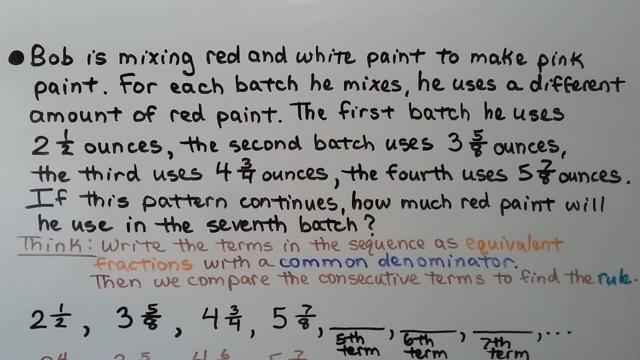 In the first batch he uses 2, 1⁄2 oz. The second batch he uses 3, 5⁸ oz. The third uses 4, 3⁴ oz. The fourth uses 5: 7⁸ oz. If this pattern continues, how much red paint will he use in the seventh batch? 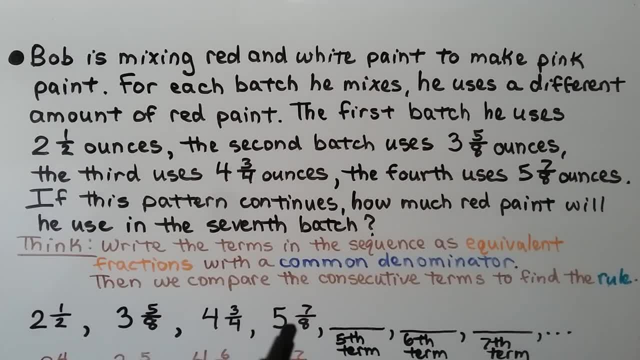 So here we've got our first batch, our second one, our third one, our fourth one- We don't know what the fifth Batch is as the fifth term or the sixth or the seventh. This is the one we really need, We think. 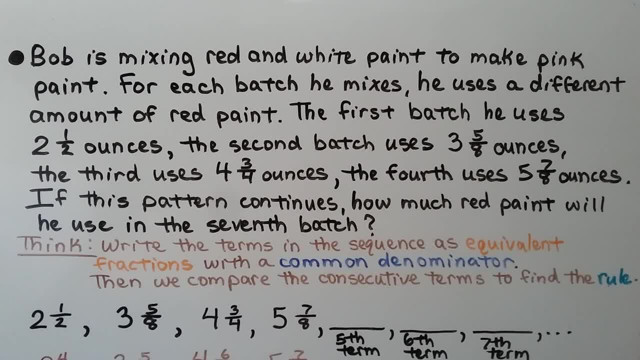 We write the terms in the sequence as equivalent fractions with a common denominator. So we have a 2, an 8, and a 4, and another 8. We can use the multiple 8 for them all to meet. Then we compare the consecutive terms to find the rule. 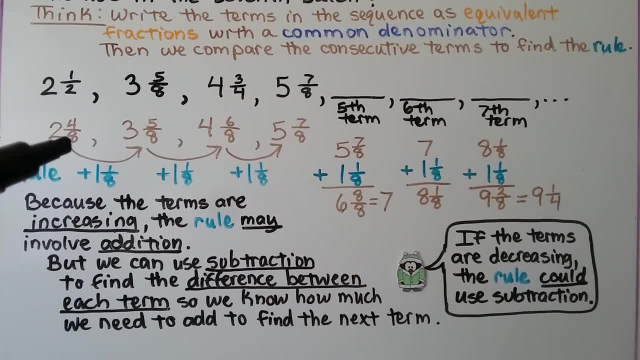 2 1⁄2,. having 8 as a denominator, we get 2, 4⁸ oz. This is already having an 8 for a denominator, so we leave that one alone. 4, 3⁴ oz would be 4, 6⁸ oz with 8 as a denominator. 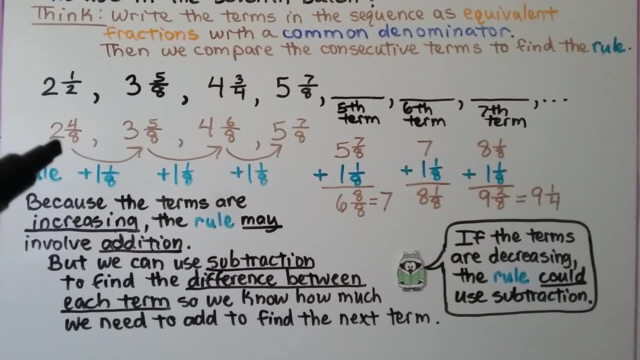 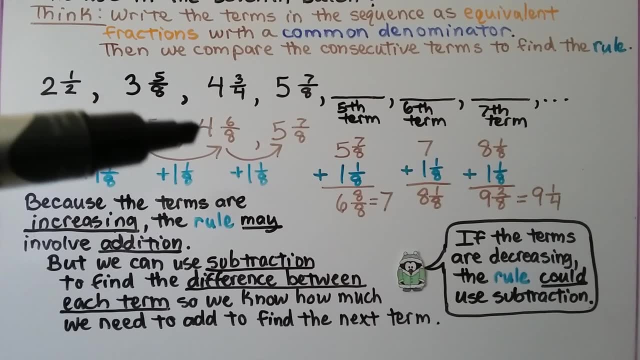 That already has an 8. So now that they all have an 8 for a denominator, a common denominator, we can find out the rule. We see: 2, 4⁸ oz, 3, 5⁸ oz, 4, 6⁸ oz, 5, 7⁸ oz. 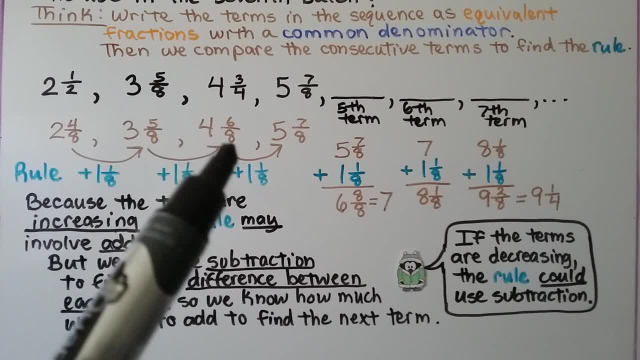 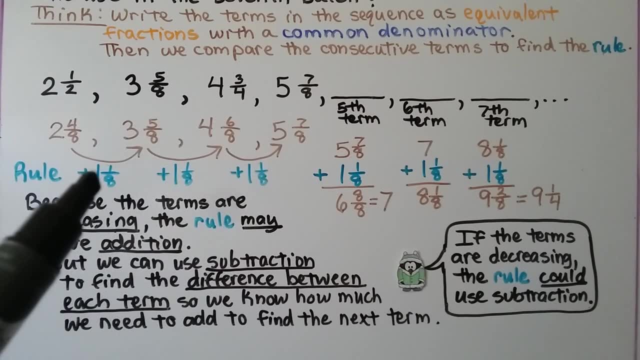 Look at what the fractions are doing: 4⁸ oz, 5⁸ oz, 6⁸ oz, 7⁸ oz. They're each going up by 1⁸, And look at the whole numbers: 2, 3,, 4, 5.. 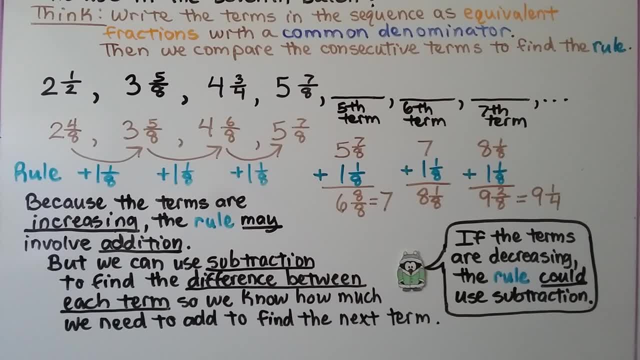 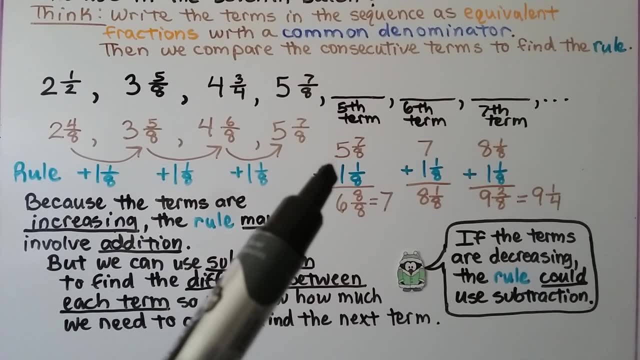 They're going up by 1.. So our rule is plus 1- 1⁸ oz. We must need to take 5- 7⁸ oz and add 1- 1⁸ oz. 7⁸ oz plus 1⁸ oz is 8⁸ oz. 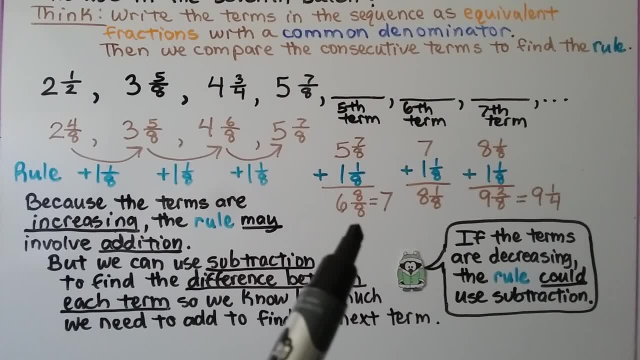 5 plus 1 is 6.. We know, when the numerator and denominator are the same, it's equal to one whole Plus 1 is 7.. This fifth term is 7.. Now we take this 7 and add 1⁸ oz. 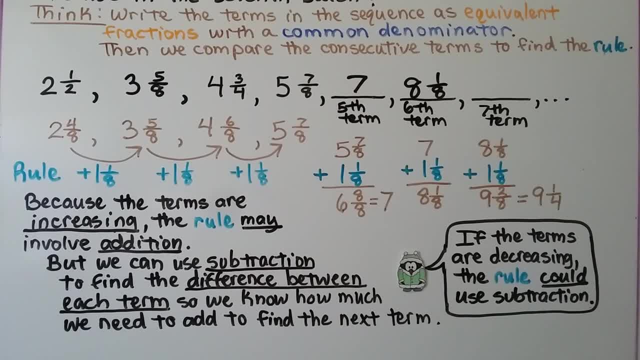 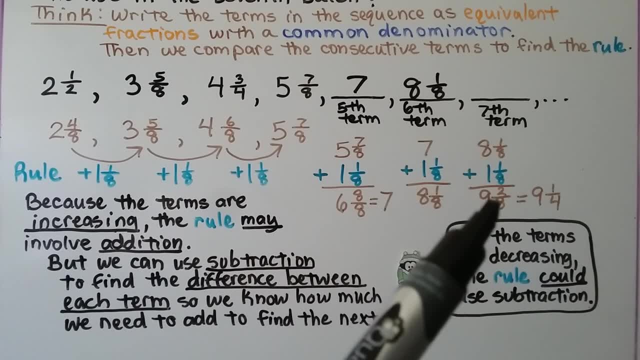 We get 8- 1⁸ oz. Now we add 8- 1⁸ oz plus 1- 1⁸ oz, We get 9- 2⁸ oz. But this is not in simplest form. In simplest form it would be 9- 1⁴ oz. 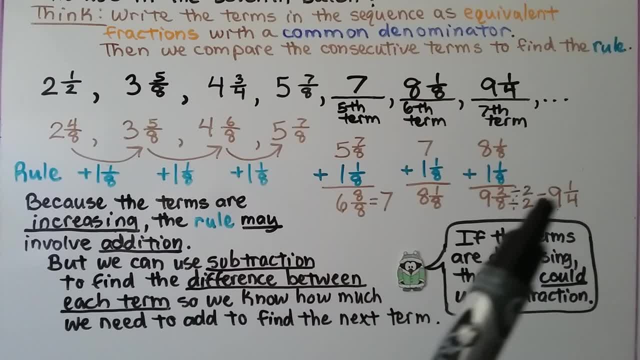 We can divide the numerator and denominator by the common factor 2.. We get 9- 1⁴ oz Now because the terms are increasing. the rule may involve addition, But we can use subtraction to find the difference between each term. so we know how much we need to add to find the term. 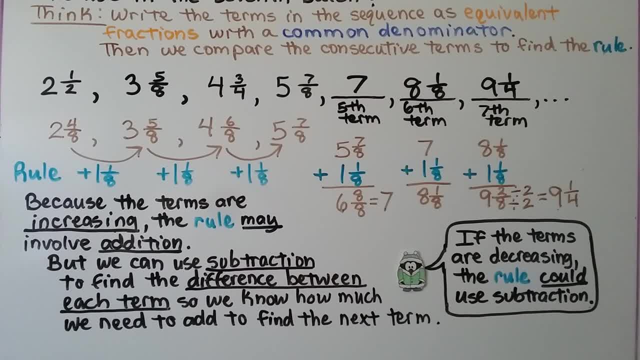 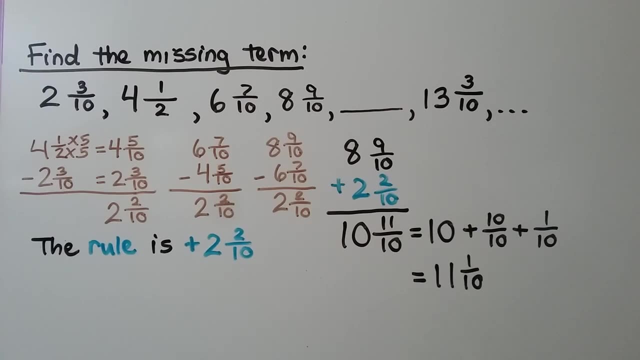 If the terms are decreasing, the rule could use subtraction. Now, if you notice, I said it may involve addition and it could use subtraction. I'll explain that at the end Here. we need to find the missing term. We have 2, 3⁰, 4 1⁄2,, 6, 7⁰, 8, 9⁰. 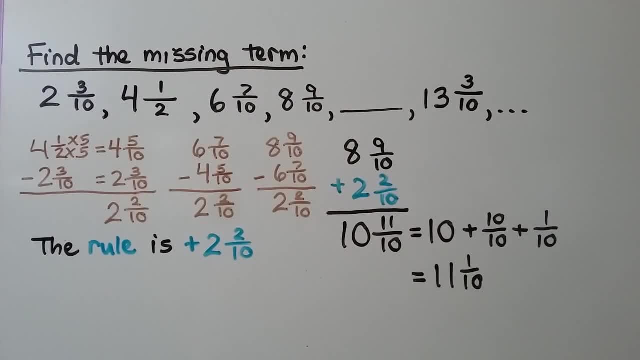 Then we have our missing term and we have 13: 3⁰. We start by doing 4 1⁄2 minus 2: 3⁰ to find the difference between them. They need the same denominator, so we're going to use 10.. 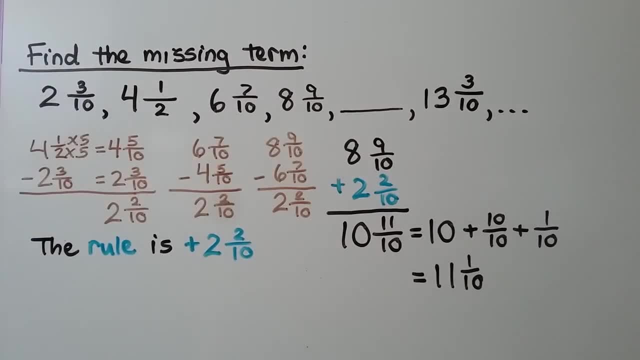 4 1⁄2 is equal to 4: 5⁰. Now we can subtract 2: 3⁰, We get 2: 2⁰. We do 6: 7⁰ minus 4: 5⁰. 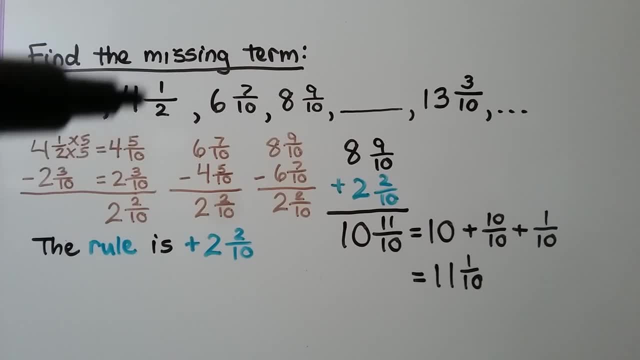 We already know that 4 1⁄2 is 4: 5⁰, so we don't need to convert it again. We don't need to change it to a common denominator. We already know that 4: 5⁰ is 4 1⁄2.. 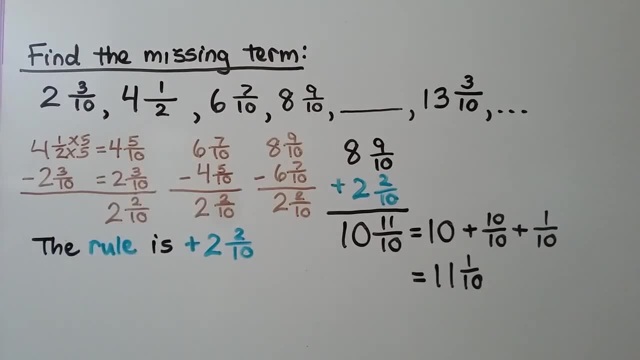 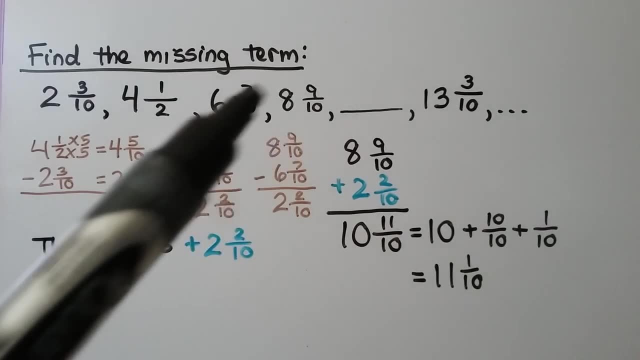 We subtract 6: 7⁰ minus 4: 5⁰, We get 2: 2⁰. So now we have two of them that are showing 2: 2⁰, But we need to check this one. We do 8: 9⁰ minus 6: 7⁰. 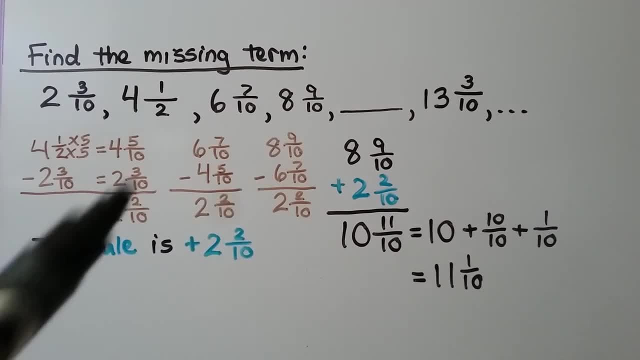 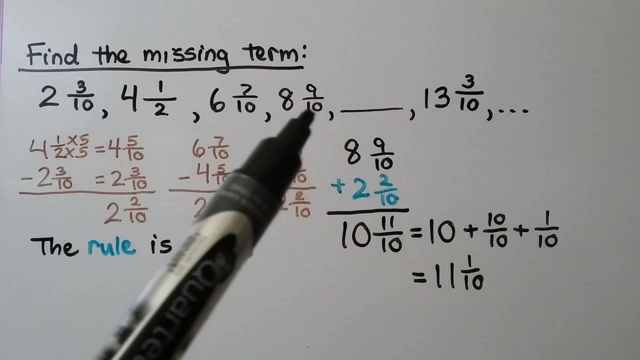 We get 2- 2⁰ again. So yes, it's very likely that the rule is add 2- 2⁰. We take this term and we add 2: 2⁰, 8, 9⁰ plus 2- 2⁰. 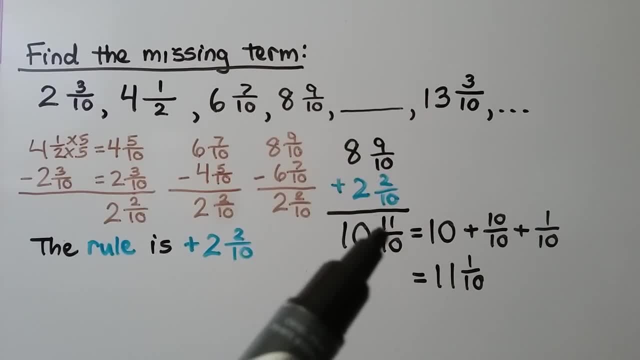 We add the numerators, 9 plus 2 is 11. We have 11⁰. We add the whole numbers and get a 10. Now we have 10- 11⁰. But this is an improper fraction. It's a fraction greater than 1 because the numerator is larger than the denominator. 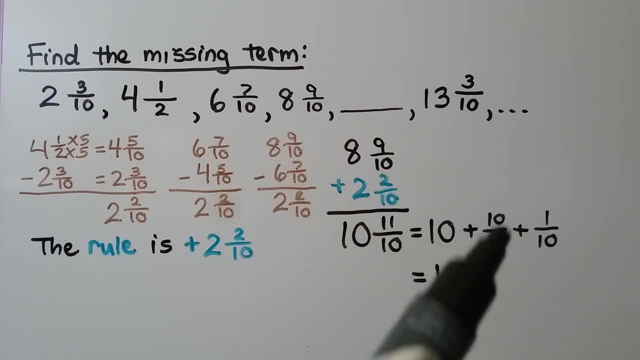 10- 11⁰ is equal to 10 plus 10⁰ as one whole plus 1⁰. We can rewrite it as 11- 1⁰. We have 10, 11, 1⁰. So we know the missing term is 11, 1⁰. 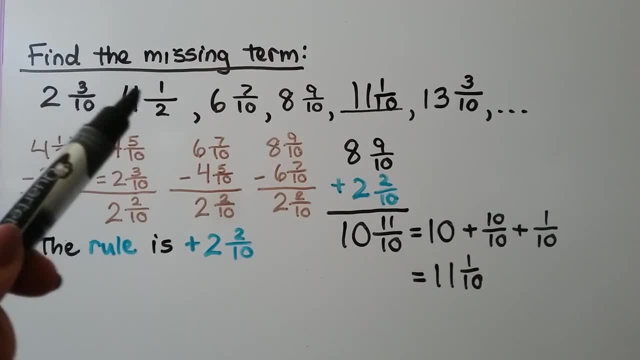 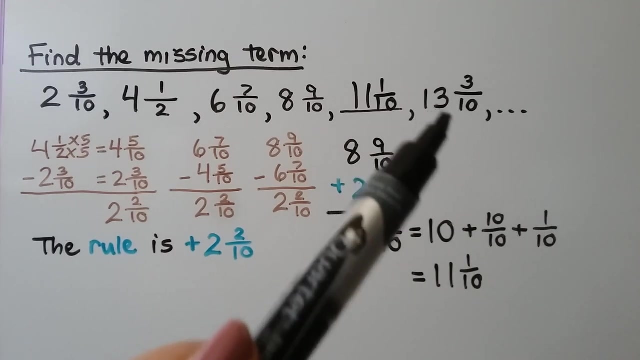 We need to use subtraction between the terms to find out the differences between them. Then, once we found this common difference, we used it to add it to this term to know the missing term. We can even check to see if 11, 1⁰ plus 2- 2⁰ is equal to 13- 3⁰. 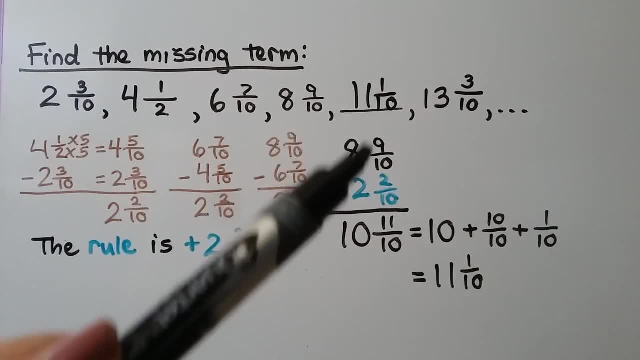 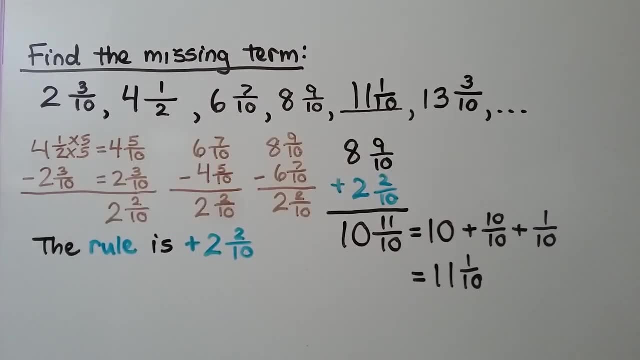 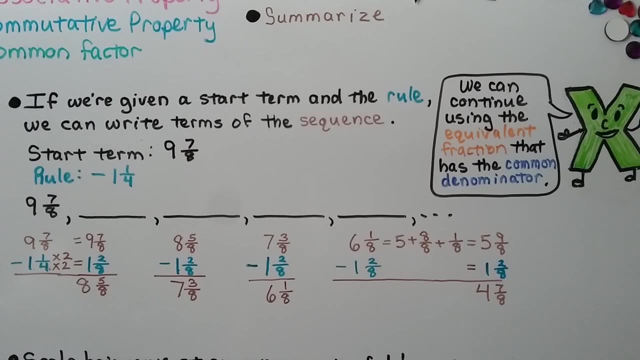 That would be a 1 numerator plus a 2 numerator. That would be 3⁰ Yep, And 11 plus 2 is 13.. Yes, 13, 3⁰. So it works for the whole sequence If we're given a start term and the rule. 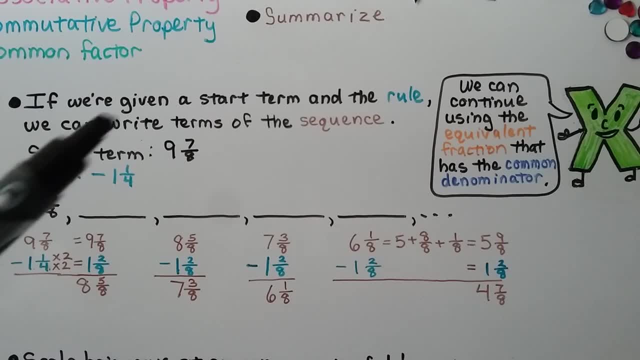 we can write terms of the sequence. Our start term is 9: 7⁰ and the rule is to subtract 1: 1⁴ And because they have different denominators, we can give them a common denominator of 8.. 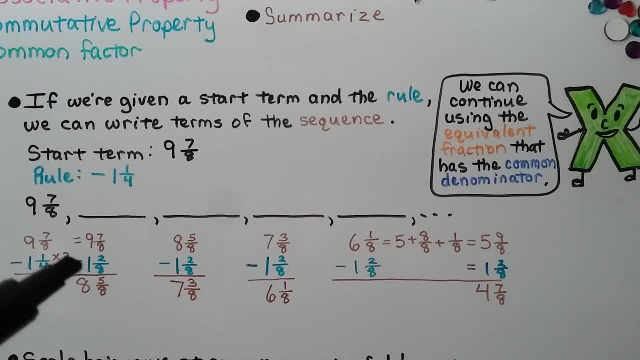 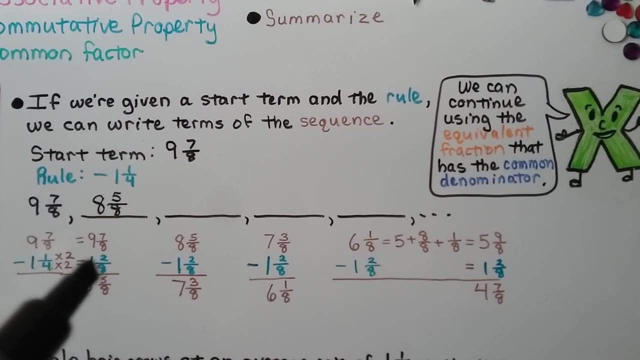 9: 7⁰ minus 1: 2⁰, That would be 8: 5⁰. We know that this term is 8: 5⁰. Now we need to subtract another 1: 1⁴, but we know we're using 1: 2⁰. 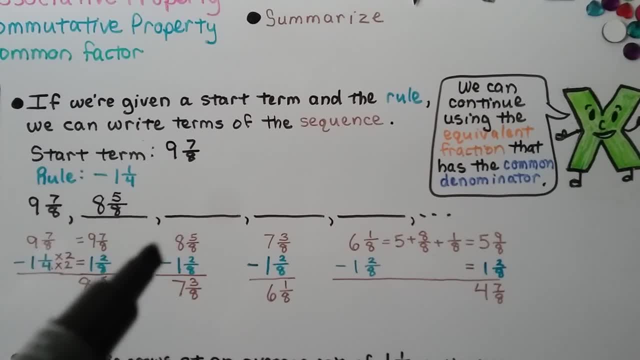 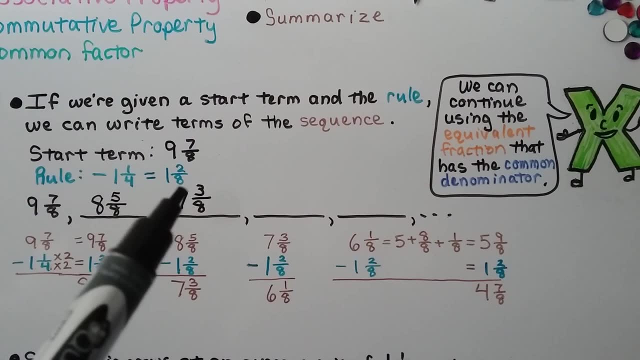 So it has the same denominator. So we have 8: 5⁰ minus 1: 2⁰, That's 7: 3⁰ for our next term. Now we have 7: 3⁰. we need to subtract 1: 2⁰. 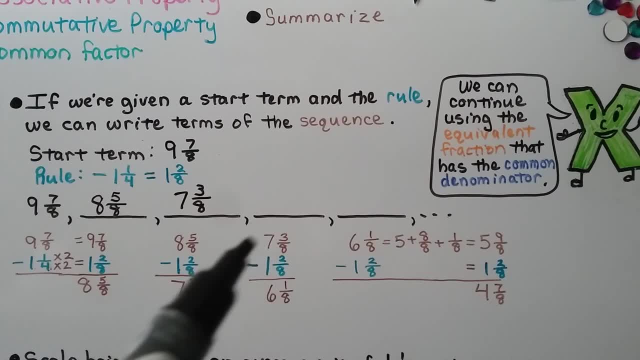 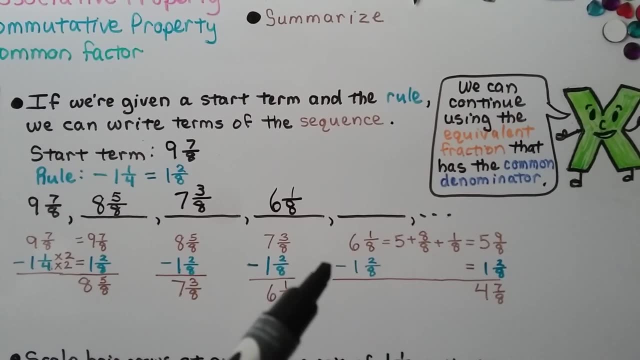 3 minus 2 is 1.. We have 1⁸. 7 minus 1 is 6.. We have 6- 1⁸. Now we have 6- 1⁸ and we need to take away 1- 2⁸. 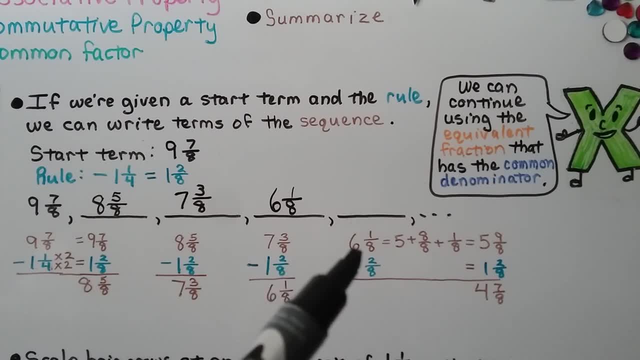 but the numerator in the minuend is not great enough to subtract the numerator in the subtrahend. We learned that in the last video We need to rename This 6. 1⁸ is equal to a 5 plus an 8⁸ as a 1 whole to make 6,. 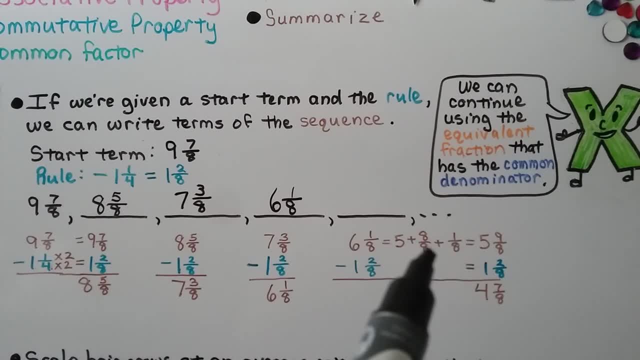 plus this 1⁸, We can add the 8⁸ plus 1⁸ to make 9⁸ and we have 5 and 9⁸. Now we can subtract 1 and 2⁸: 9 minus 2 is 7.. 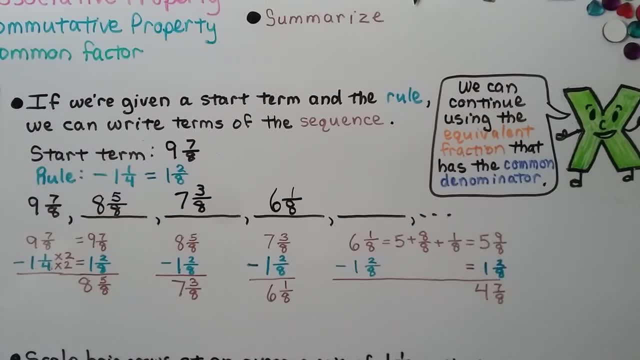 We have 7⁸, and 5 minus 1 is 4.. We have 4 and 7⁸ for the next term. So if what I did here really confused you, you need to look in the description for video 6.6 and watch that one real quick. 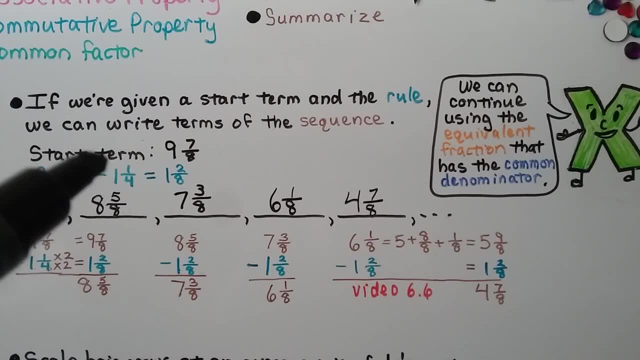 So do you notice how it said the rule was to subtract 1 and 1⁴, but because we needed eighths, we found it was 1 and 2⁸, and then that's what we used for the rest of our math. 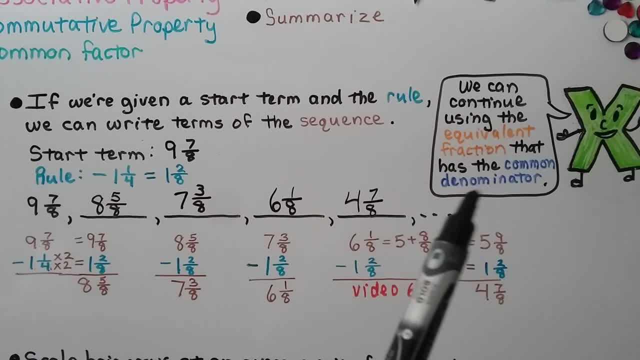 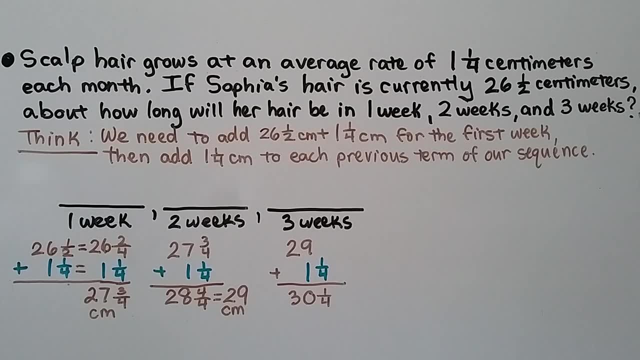 to find the next term in the sequence, So we can continue using the equivalent fraction that has the common denominator Scalp. hair grows at an average rate of 1 and 1⁴ centimeters each month. If Sophia's hair is currently 26 and 1⁄2 centimeters, 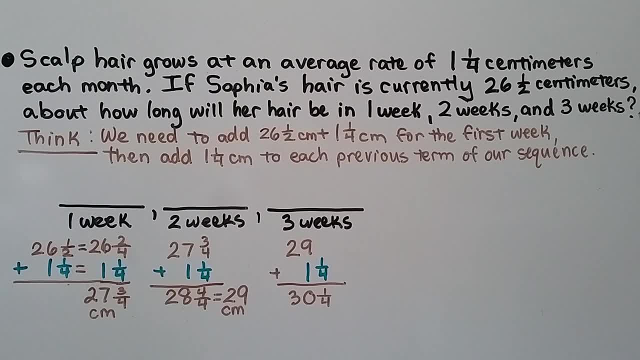 about how long will her hair be in one week, two weeks and three weeks? So we think we need to add 26 and 1⁄2 centimeters plus 1 and 1⁴ centimeter for the first week, Then add 1 and 1⁴ centimeter. 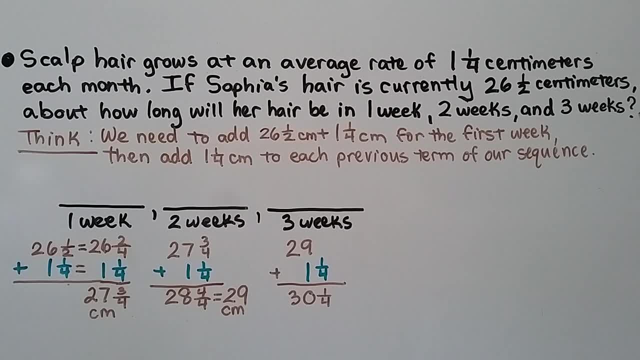 to each previous term of our sequence. So we have 26 and 1⁄2 plus 1 and 1⁴. They need the same denominator, so 26 and 1⁄2 is the same thing as 26 and 2⁴. 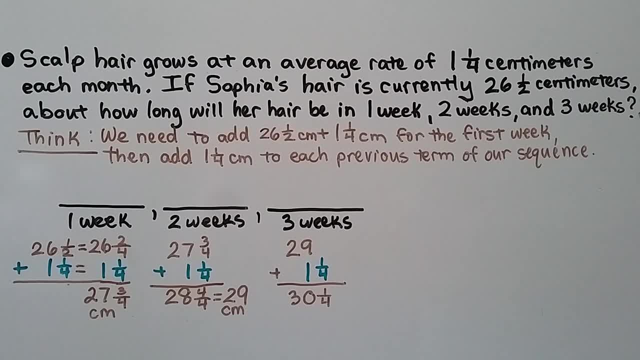 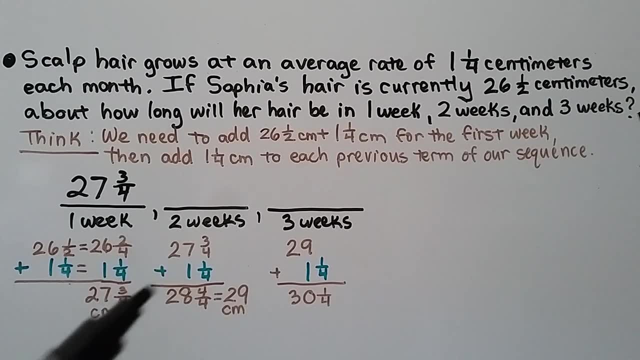 We get 27 and 3⁴ centimeter after one week. For the second week, after two weeks, we need to add the 27 and 3⁴ plus another 1 and 1⁴. 3 plus 1 is 4.. 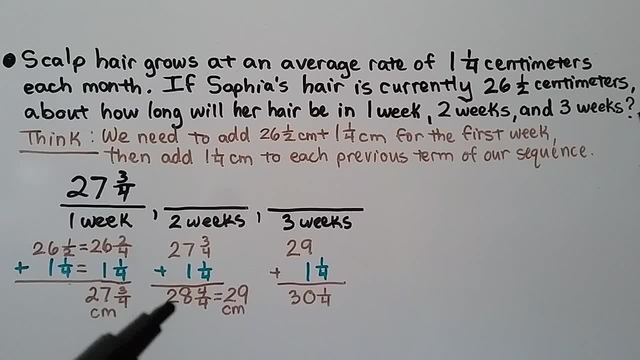 We get 4⁴. 27 plus 1 is 28.. We have the same numerator and denominator, so that's equal to one whole. We have 28 plus 1⁴, That's 29 centimeters. For the third week after three weeks, 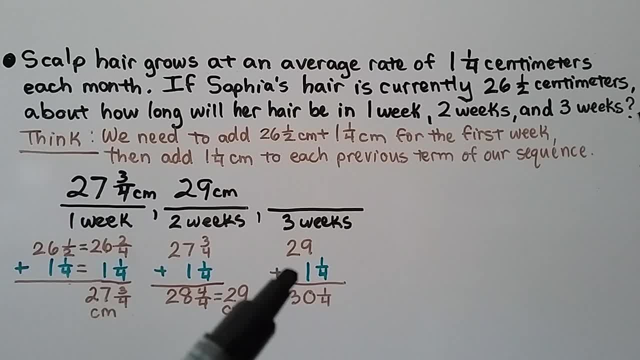 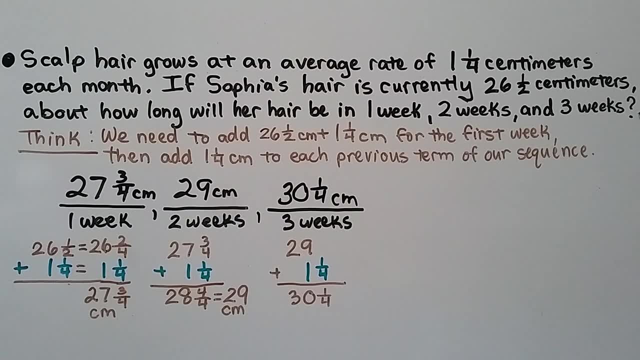 we just need to add this 29 centimeters to 1 and 1⁴ centimeters, We get 30 and 1⁴ centimeters, And if Sophia didn't cut her hair and it continued to grow at this rate, we would be able to tell you how long her hair would be. 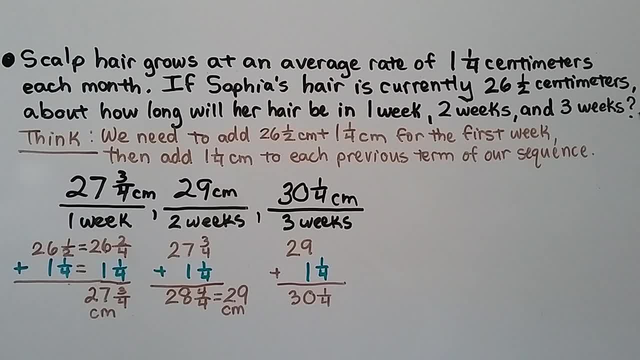 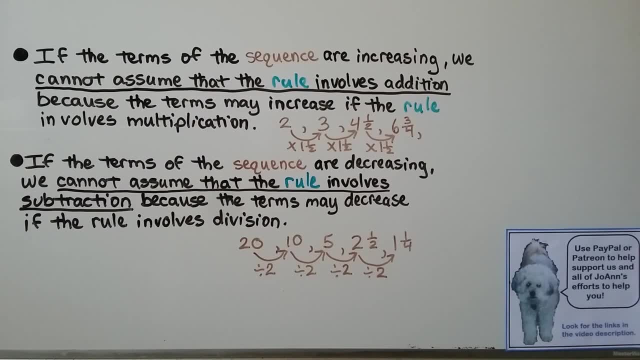 in 12 weeks or 20 weeks or 30 weeks or more. So, as I said before, if the terms of the sequence are increasing, it could involve addition. This is why, if the terms of the sequence are increasing, we cannot assume that the rule involves addition. 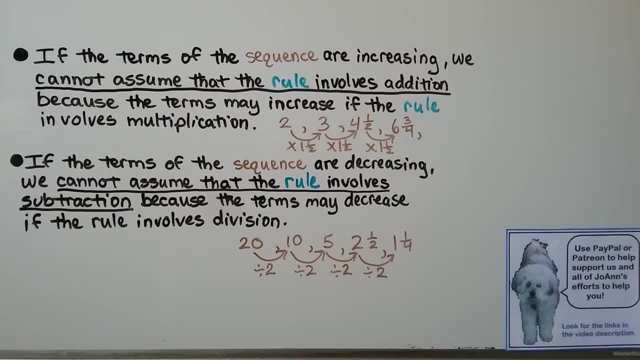 because the terms may increase if the rule involves multiplication. If we have 2, then 3,, then 4 1⁄2, then 6, 3⁴, the rule could be multiply by 1 1⁄2.. 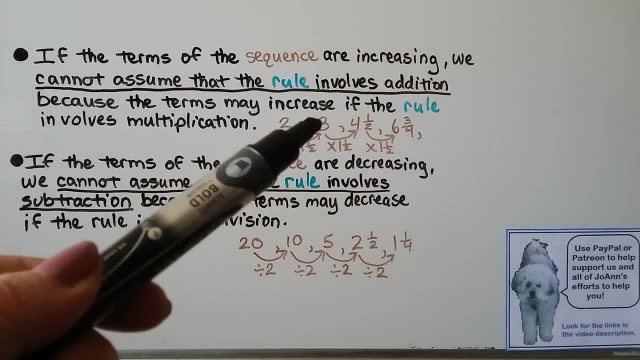 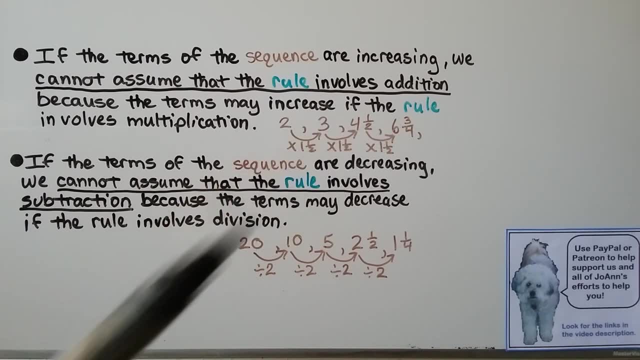 If we have 1 1⁄2 two times, it's equal to 3.. And if we do 3 times 1 1⁄2, we'll have 4 1⁄2.. And if we do 4 1⁄2 times 1 1⁄2, we'll have 6, 3⁴. 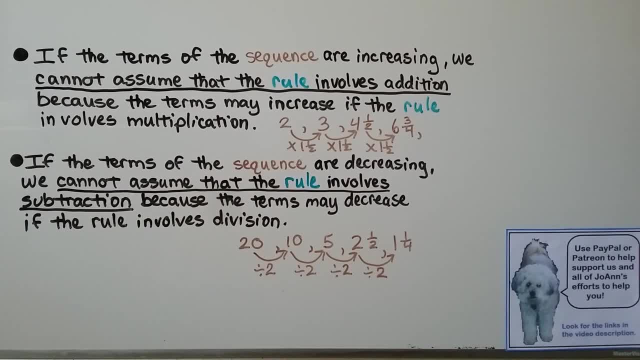 So it's increasing, but it's not using addition. So that's why it says it could be addition if it's increasing And if the terms of the sequence are decreasing, we cannot assume that the rule involves only subtraction, because the terms may decrease if the rule involves division. 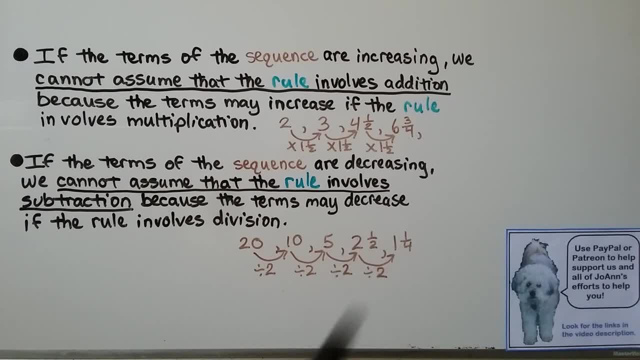 Here we have a 20, then a 10, then a 5, then a 2 1⁄2, then a 1: 1⁴. They are definitely decreasing, but what's happening is we have 20 divided by 2, which is 10,. 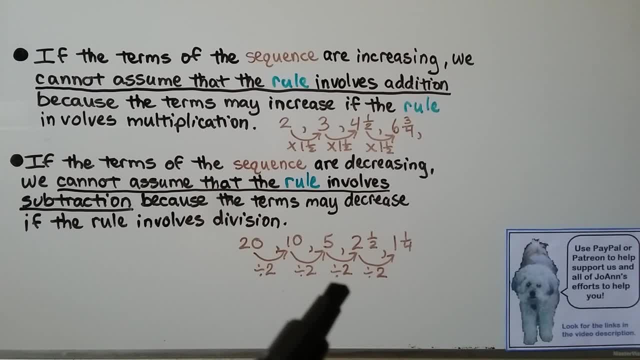 10 divided by 2, which is 5,, 5 divided by 2,, which is 2 1⁄2,, 2 1⁄2 divided by 2, which is 1, 1⁴, So it's decreasing and it's not using subtraction. 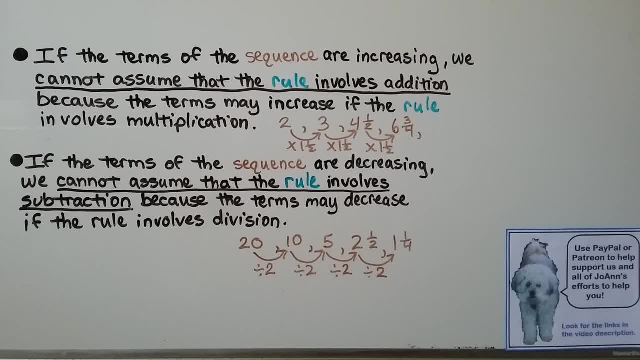 It's using division, So be very careful. It's not definite that it's addition if it's increasing and it's not definitely using subtraction if it's decreasing. Okay, Remember that you can click this description for the previous helpful videos, like the patterns with decimals of 3.10.